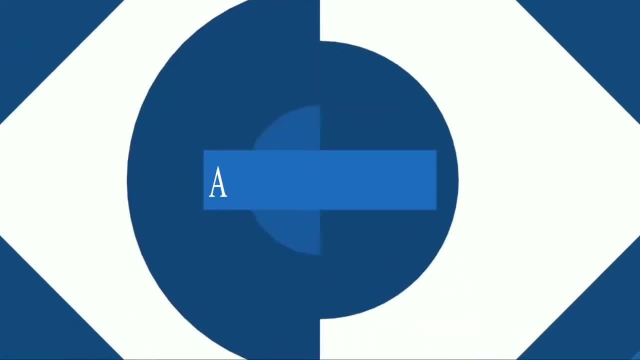 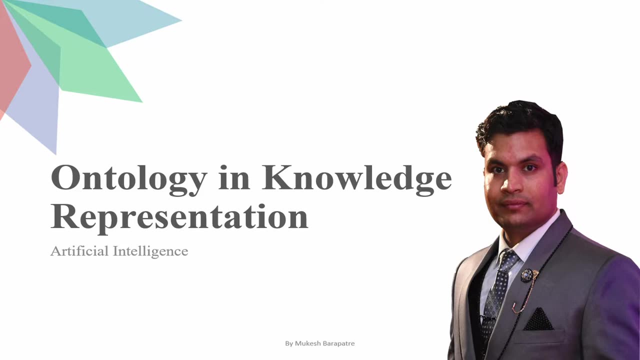 Hello friends, welcome to the video series of artificial intelligence. My name is Mukesh Bharapatra. Today we are going to learn ontology in knowledge representations. So let's get started. In today's lesson we are going to discuss ontology Now. first question is that: 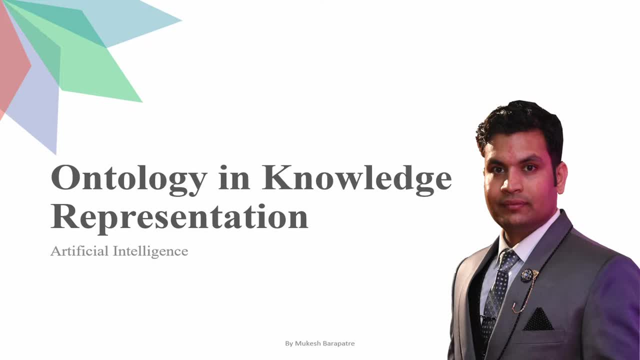 what is ontology. Ontology is in computer science and information science, and ontology encompasses representations or formal naming and definitions of categories, properties and relations between the concepts. Whatever we are going to represent our knowledge, in our database or in our artificial intelligence machine, we required the representation scheme, or we also 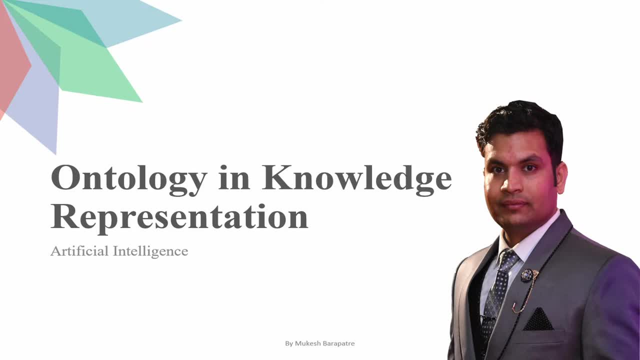 required some formal naming, definitions and categories. So this is that concept is nothing about the ontology. It is a branch of computer science where we deal with the representations of knowledge or information into a machine. The question is: ontology? Ontology means what? Ontology means that in a philosophical way, if we look at our data or whatever information, 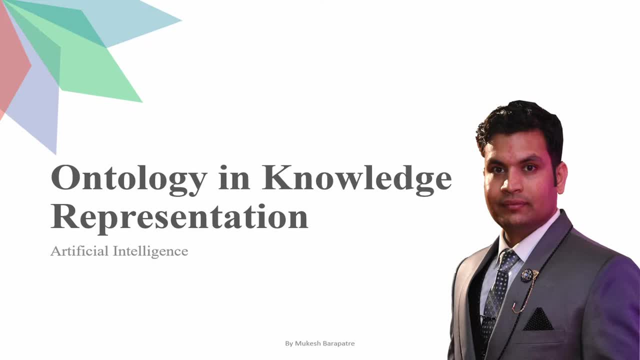 we want to store or we want to capture, then at what level or with what detailing or category will you store that information? So those things that come under your knowledge, representations, your code or courage. we have to have an ontology type of knowledge and it is a philosophical term where we have different. types of knowledge, different formal naming and conventions. So how do we gain events and the relationships between objects and concepts, from services to the organisms and entities The data are stored in our machines are domain specific knowledge in which this information can be stored. So if you are looking for environments where the information can be stored, then needless. to say how to store this information So that蚝äuä vai šäätu can kadın processes from human correctly've found region go, & woman's nature is none other that not suppose to do it or not come tomons or 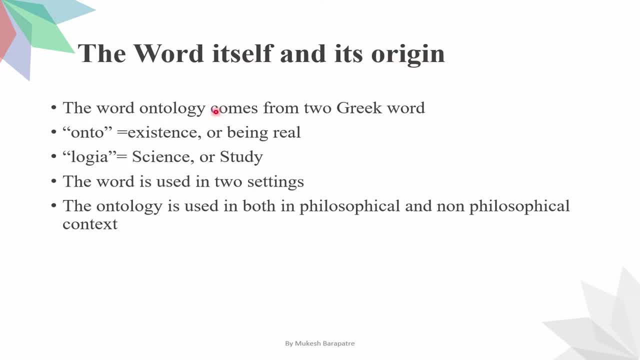 ontology, the word itself and its origin. the word ontology comes from the two greek word. first one is onto. that is also called as existence or being real. okay, we will explain what is the onto and what is a logia. okay, so second word is logia. it's nothing about the science or a study. 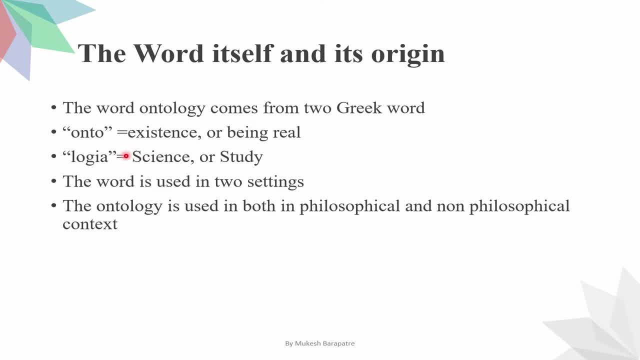 so that means ontology is nothing about the study of existence or a being real. the word is used in two settings. first one: ontology is used in both philosophical and non-philosophical context. we are we are not concentrated on the philosophical word, we are going to concentrate on non-philosophical 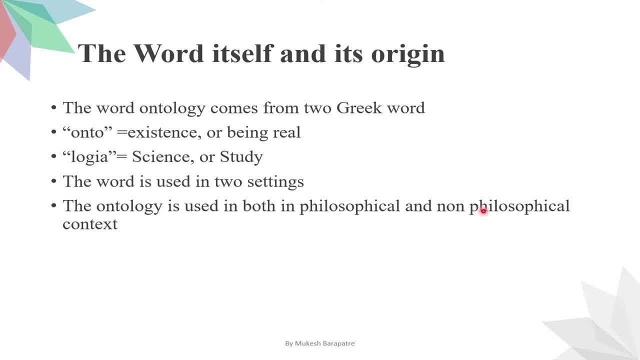 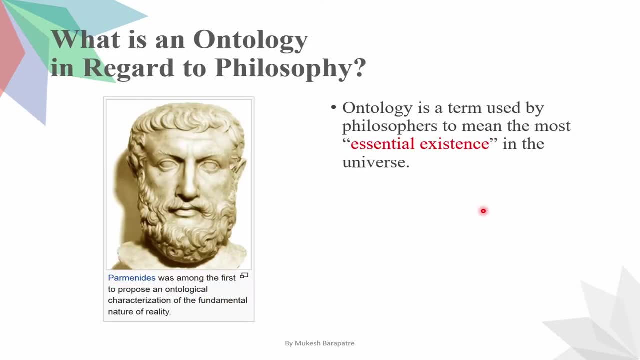 context, that is, in a computer science. here we are learning the knowledge representations. that why we use ontology in context of knowledge representations. what is ontology in regards of philosophy? ontology is a term used by philosophers to mean the most essential existence in the universe. philosophical or philosophers believe that, for example, we have a life. 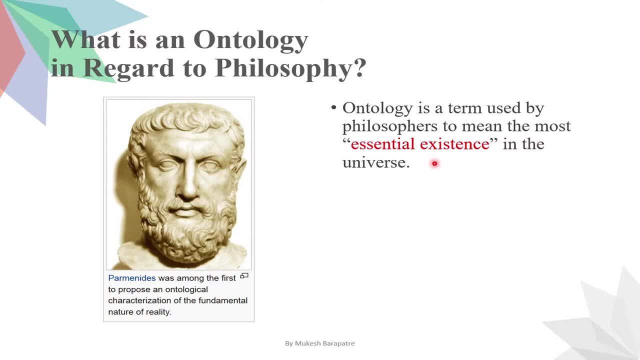 there is a life in humans, there is a soul according to which the human being works. so that is the philosophical word. we can say that the soul in the human being. now, if we study in the soul, then the life in it. if we study in detail, then what is its existence, what is its detailing, what is its? 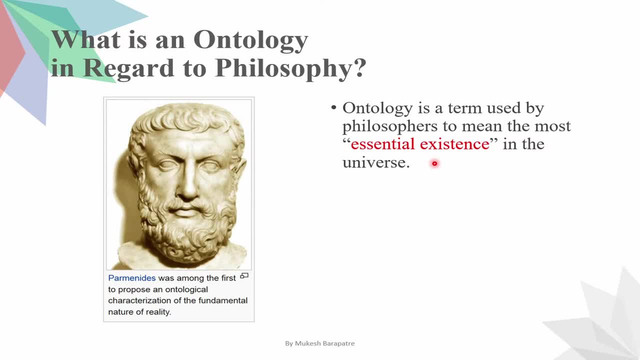 identity, that society, of which person has served humans, is going to have the chance to come alive. maybe they will come to us also. how many of us will be alive? how many of us will be taking birth at that age? we are like a child. that is one kind of a house for us. 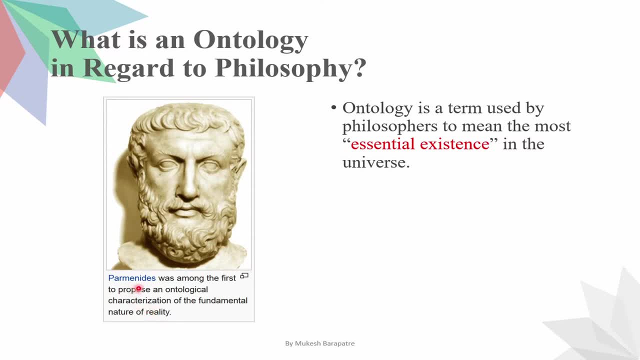 we can make love to them, we can make diürdam or we get a good child. this will give us a lot of a audacity. this is about this, all these questions which are connected by philosophy, and then these: If we want to do a detailed analysis of a concept or a category, then how can we categorize it or make a list of it? 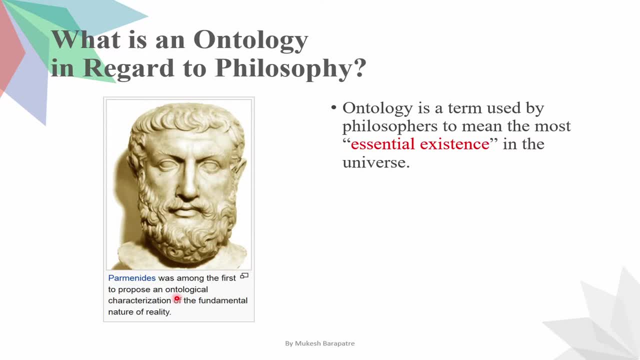 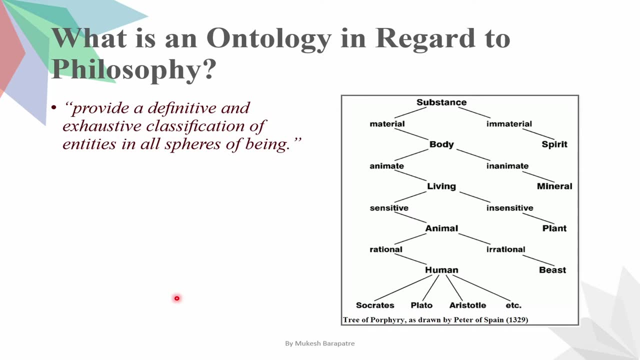 That is nothing but a philosophical word, and we can call it our own philosophy. So what is an anthology in regards to a philosophy To provide the definitive and exhaustive classifications of entities in all spheres of being? That is, how can we represent anything in our environment in a philosophical way? 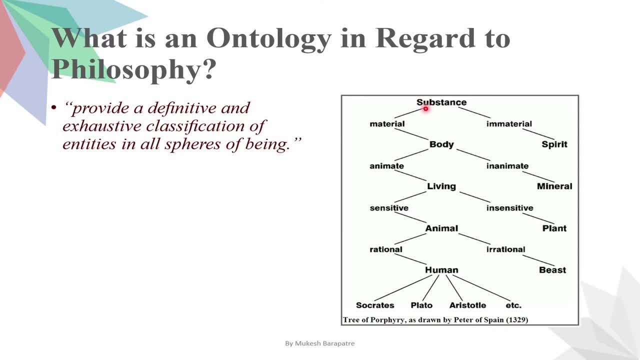 For example, we have a substance. If we classify it in substance, then we get the materials and immaterials. So in immaterials we get spirits, In materials we get our body. So we have a body. 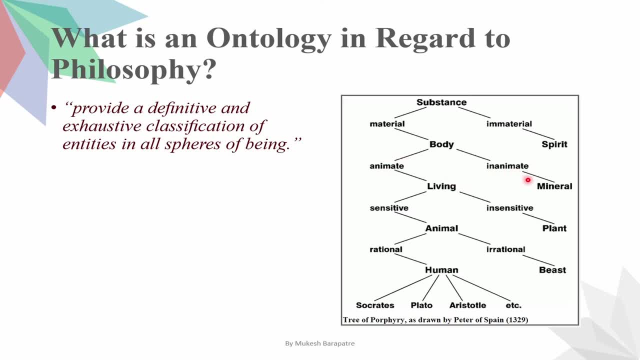 Inanimated. Inanimated means that which does not have life. it will come in minerals, In our body, which has life- we call it animated- In which living things come. there will be sensitivity and insensitivity, Which we call plants. 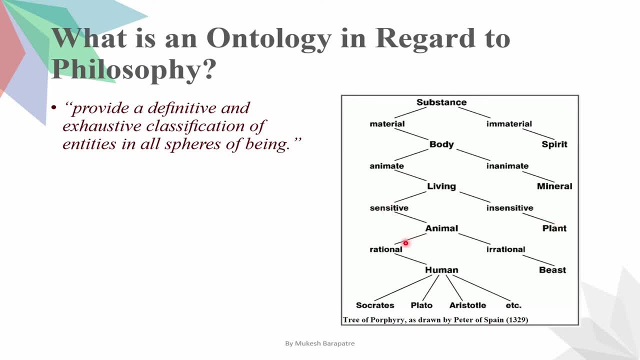 In sensitive materials. our animals come In animals. there are some relationships, So it will come in human being characteristics. What we are doing is we are categorizing and classifying our data in different entities and different objects. That is nothing but our own ontology. 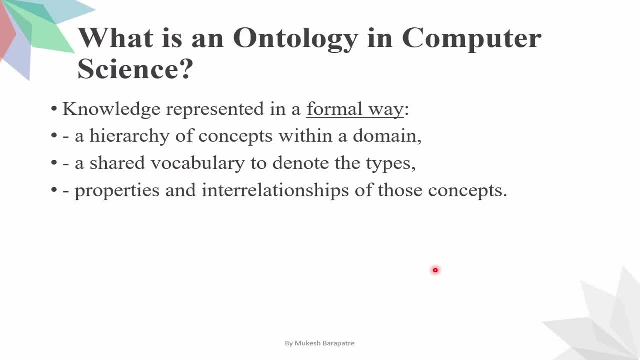 What is an ontology? It is an ontology in computer science, That is, knowledge representation in formal way. How will we use our ontology in knowledge representation? A hierarchy of concepts within a domain, That is, whatever information or knowledge we have to store in knowledge base in artificial intelligence. 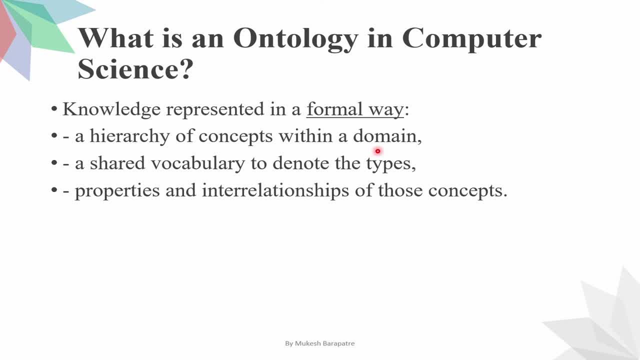 we have to create a hierarchy of that concept so that we can store it properly, A shared vocabulary to denote the types, Different categories, different entities, Their naming conventions- All these things will be used here- Properties and interrelationships of those concepts. 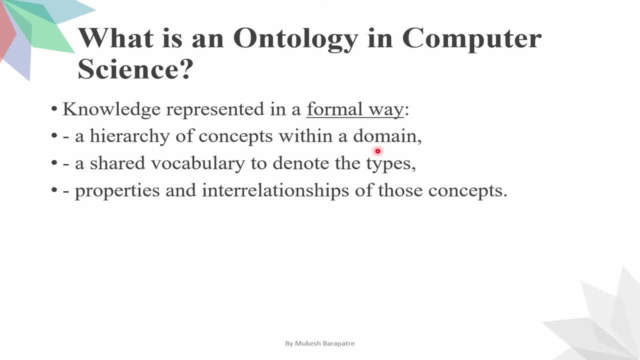 All the entities and objects that we have, the relationships between them, we have to represent them through ontology or within the concept of ontology. So this is nothing but the ontology in knowledge representation. That is what is an ontology in computer science. 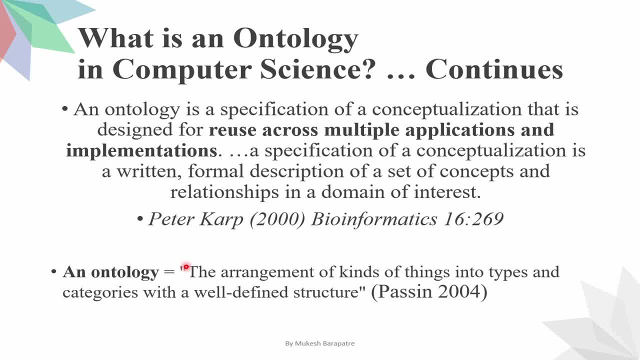 An ontology is a specification of conceptualizations that is designed for reuse across multiple applications and implementations. A specification of conceptualization is written formal descriptions of a set of concepts and relationships in a domain of interest: Peter Karp 2000.. It is a small term. 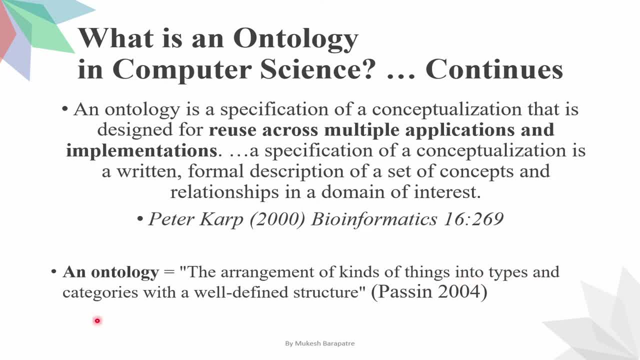 The arrangement of kind of things into a types and categories with a well-defined structure. That is passing in 2004.. Simply, If we look at the context of knowledge representation- whatever knowledge we have- we insert that data into a database or knowledge base. 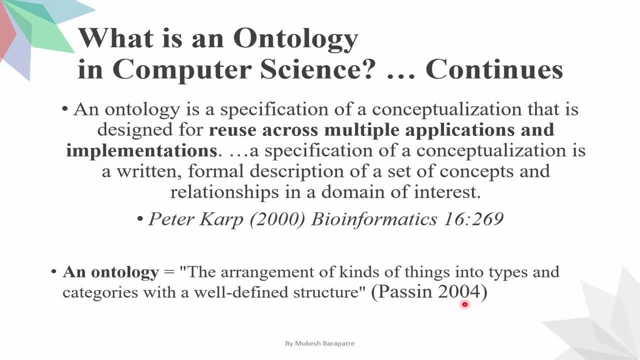 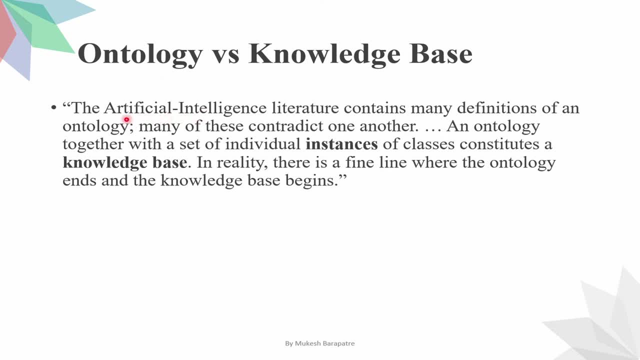 So we have to properly arrange that knowledge in a well-defined structure. So that term is called as ontology, Ontology versus knowledge base. The artificial intelligence literature contains many definitions of ontology. Many of these contradict one another And ontology together. 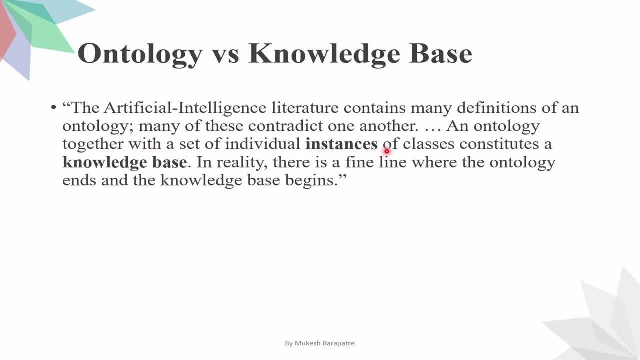 with the sets of individual instances of a class constitute a knowledge base. In reality, there are a fine line where the ontology ends with the knowledge base begins. We have to differentiate what is ontology and knowledge base. In ontology it is a philosophical term. 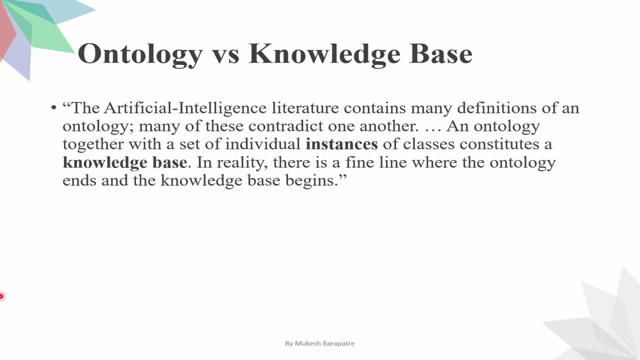 Where we are going to extract the data or knowledge or information, and we have to set it into a well-defined structure. Okay, So that is nothing about the ontology. What happens in ontology is that whatever knowledge you have, you have to organize it properly and keep it in a proper way. 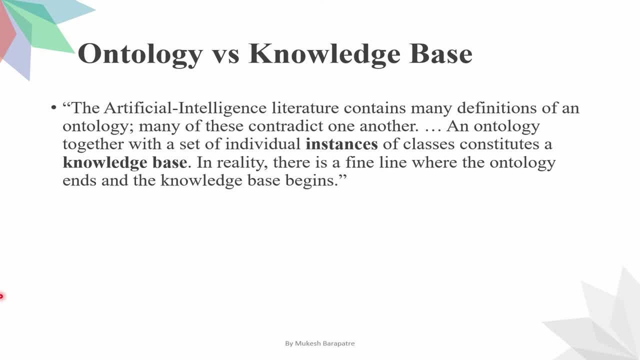 What happens in knowledge base is that whenever we want to store data in a machine again, we have to do different categorizations and classifications here: Objects, properties, attributes, hierarchy, plus relationships- all these information we have to store. So there is only this much difference between ontology and knowledge base. 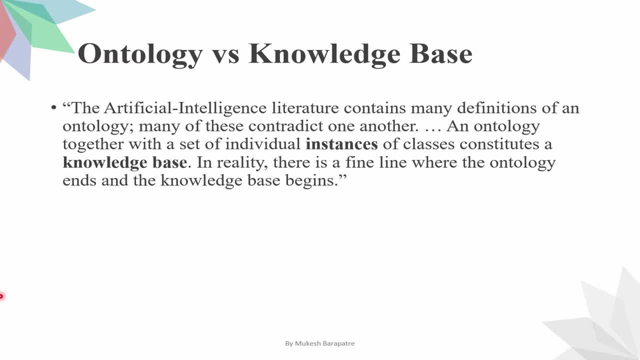 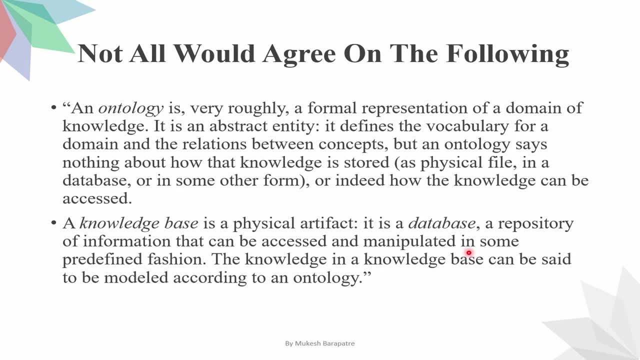 So it is a philosophical word And knowledge base is a real term. This is a real term word Where we will store knowledge in the database. Not all would agree on the following: An ontology is a very roughly a formal representation of domain knowledge. 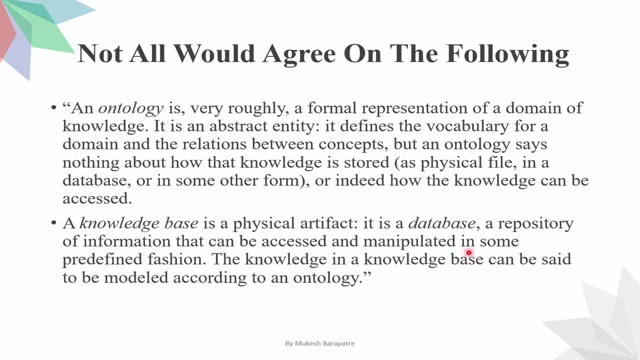 An ontology is very roughly a formal representation of domain knowledge. It is an abstract entity. Yes, So what is ontology? You do formal representations of domain knowledge, So it is an abstract entity Here, whenever you do an abstract entity, 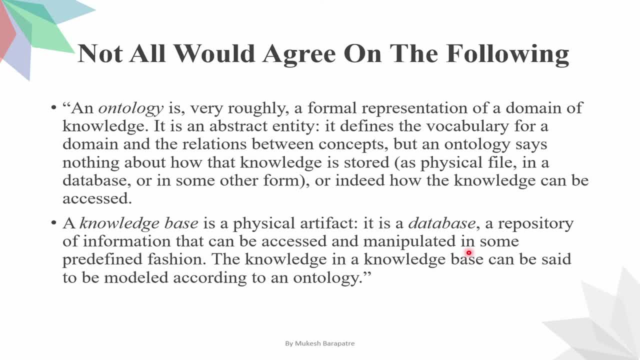 you will understand that what is the meaning of detail and what is the meaning of abstract. So it defines the vocabulary for the domain and the relationship between the concept. But an ontology says nothing about how the knowledge is stored: A physical file, in a database or in some other forms. 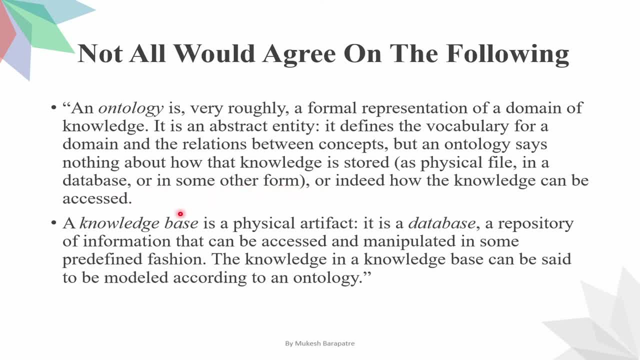 Or indeed how the knowledge can be accessed. The knowledge base is a physical artifact. It is the database, The repository of information that can be accessed and manipulated in some predefined fashions. The knowledge in the knowledge base can be said to be modelled according to the ontology. 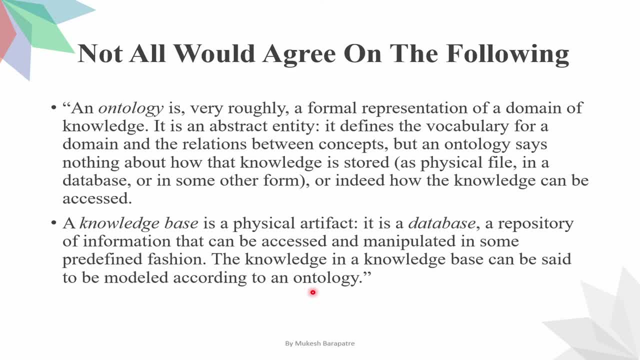 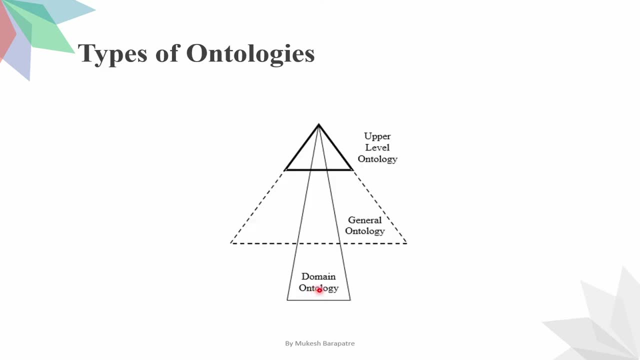 But this is the abstract term. Ontology is an abstract term where we have to represent the data, But knowledge is a physical term where we are going to store the knowledge into a database. Types of ontology: We have three types of ontology. That is, upper level ontology. 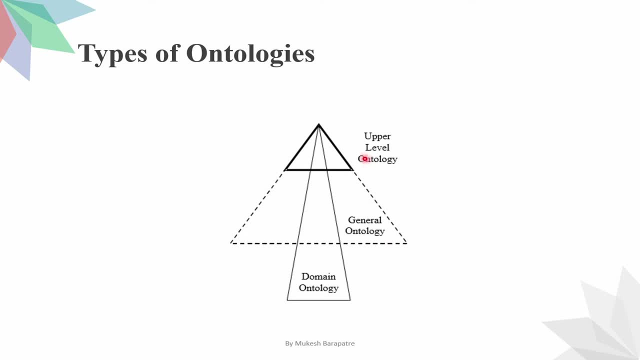 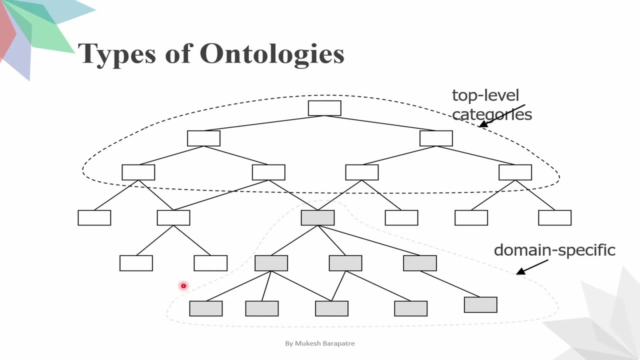 general ontology and domain specific ontology. Now, what is upper level ontology? We will explain with the help of some examples. Let's suppose we have some classifications or we have some informations, So that roughly informations, that top level informations, are stored. 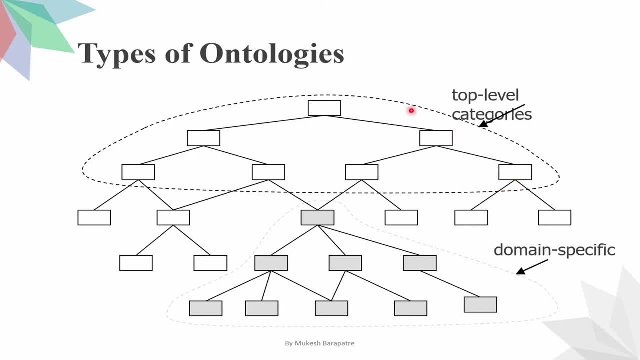 Top level categories are called as upper level categories or upper level ontologies. Generalized ontologies, which is in between this And domain specific ontology, means the informations which is regarded to only a domain, So that is called as domain specific ontology or domain specific knowledge. 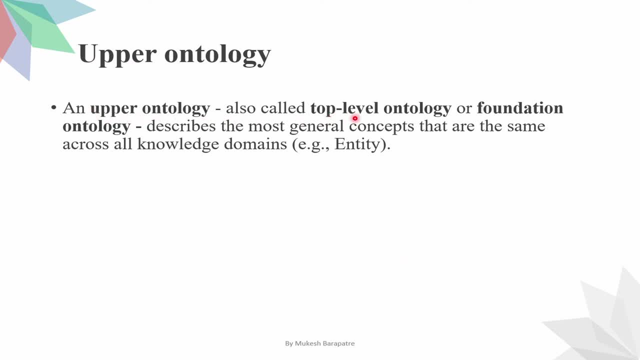 Upper ontology. The upper ontology is also called as top level ontology or foundation ontology, Which describe the most general concept that are same across all knowledge domain. For example, if I talk about any information, then all the type of domains have different knowledge. 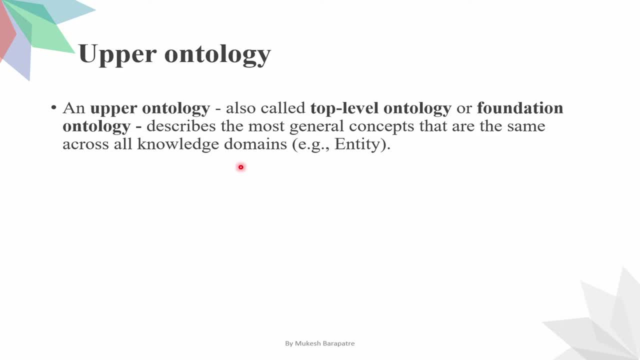 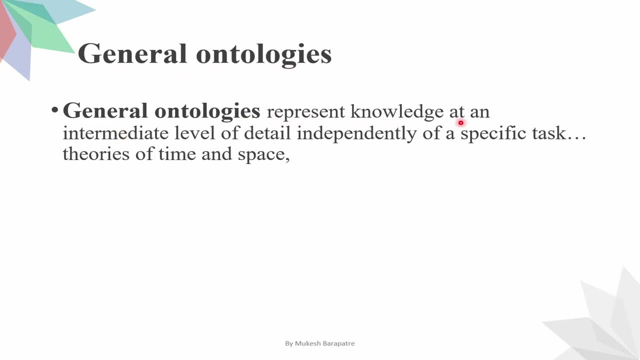 And all the domains have same type of knowledge. So that type of information is called as upper level ontology. Now talking about the general ontologies. General ontologies represent the knowledge at the intermediate level of detail, Independently of the specific task theories and the time and space. 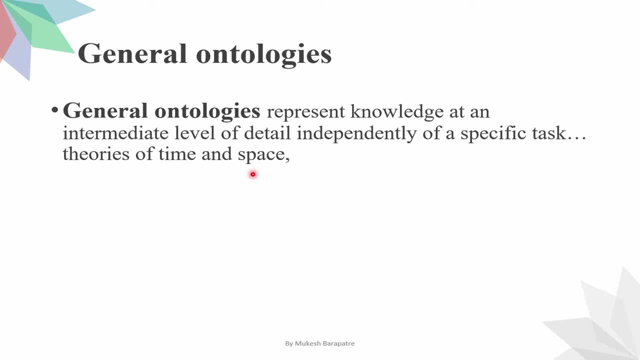 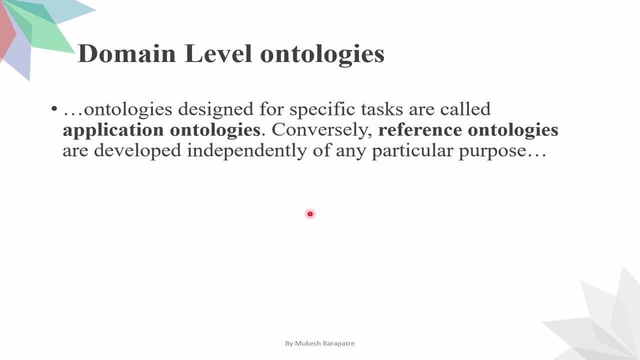 Means whatever information you have, the details of intermediate level comes under the general ontology, Domain level ontologies. For example, if we have any specific information, specific domain, we have to extract the information or detailing of any specific domain, So that particular type of detailing or representation is called as domain ontologies. 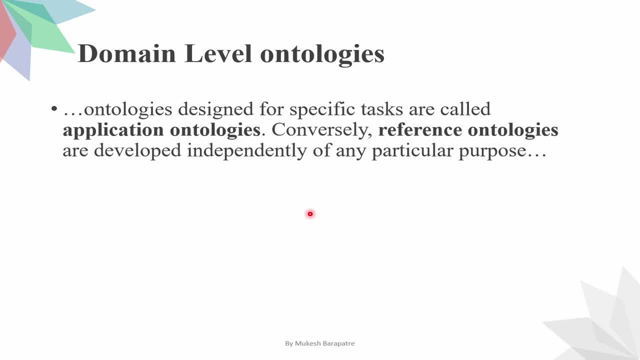 Example: if we are gathering the knowledge or extracting the knowledge from the doctors, If we have to extract the knowledge in the brain of the doctors and store it in the knowledge base, then we are talking about that specific doctor. So here we have three types of levels. 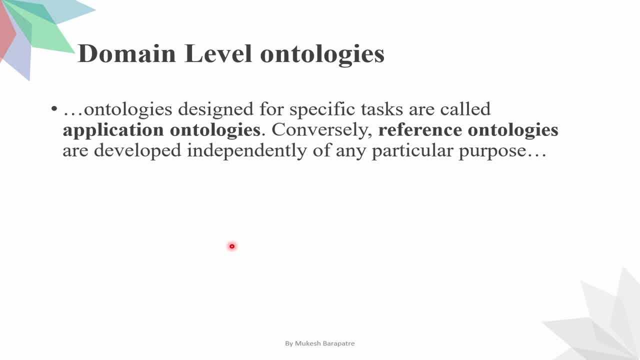 First one is upper level. Second one is general level. Third one is domain level. Domain level means the knowledge that we are going to get for that specific reference or specific application. How we are going to develop that knowledge, How we are going to develop its formal definitions. 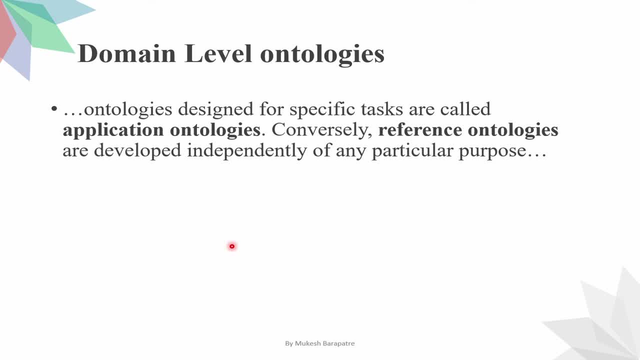 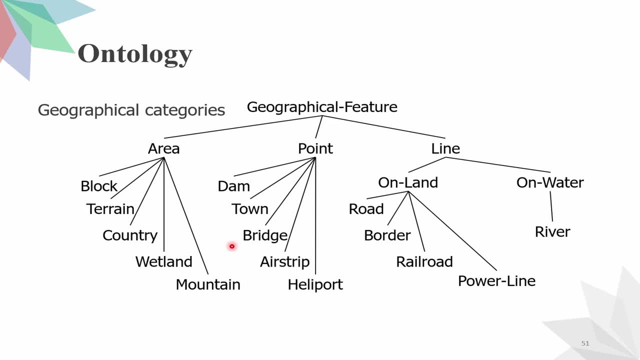 How we are going to develop its representations. That is, Let's see in the example, For example, Geographical categories. If I talk about any geographical categories then it has some features: Area, Point and Line. Okay, If I talk about area specific, 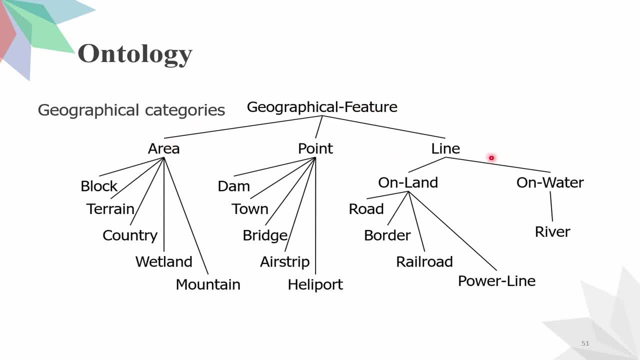 So the area, point and line in the geographical features. So these are called as top level or upper level ontology. These are called as top level or upper level ontology. Okay, In specific or domain level ontologies, area that will contain block terrain, country, wetland, mountains. 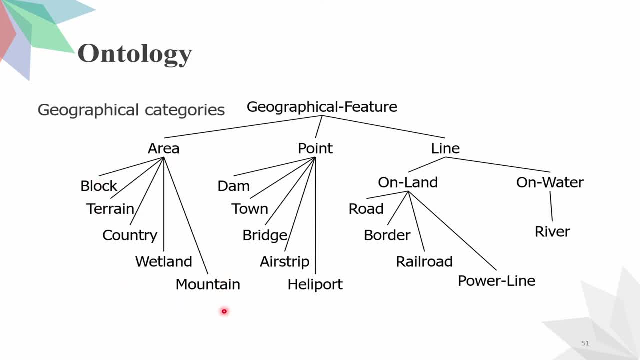 So according to area, we have some of these specific types. Okay, If we are talking about the terrain, a specific domain means if I talk about the terrain, then here some details of terrain will also come out. So that type of called as domain specific information. 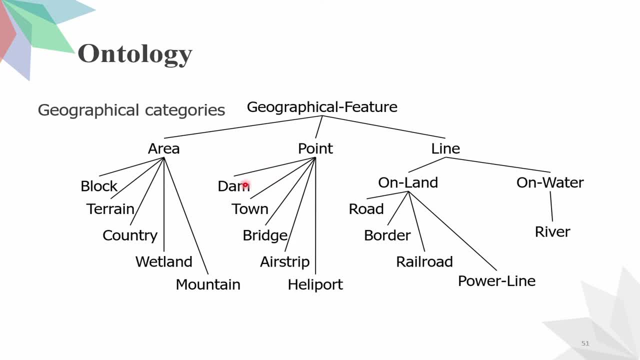 Point, point in a point. we have a dam, town, bridge, airstrips, heliport. So these are the different general level ontologies. If I talk about heliport, then heliport will be domain specific ontology. 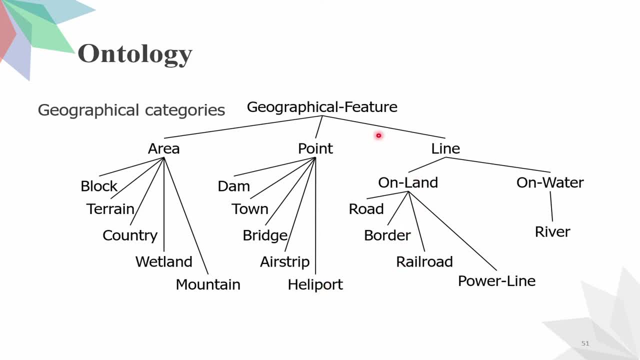 Domain specific knowledge will be there. So in the same way, our example will run, Similar example. if I tell you by representing, then we have education system. Education system is nothing about the top level. Now in education system, many streams run. 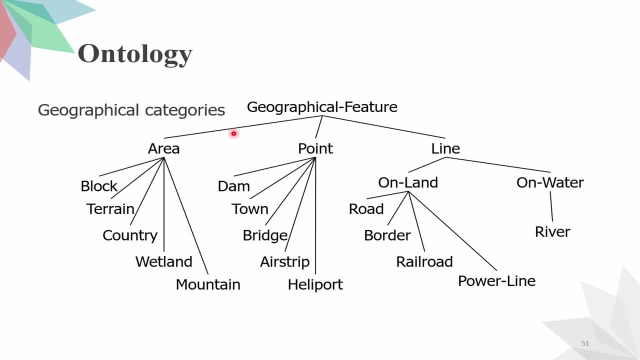 For example, your engineering came medical came your BSc, BCom. So these are the upper level or top level ontologies. Here your top level information is there by which you can relate specific information and represent it. Now let's come to the general level. 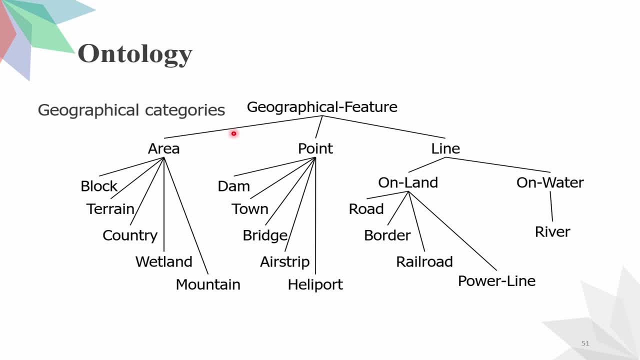 If we come to the general level, then let's suppose we have considering the engineering field. In engineering field we have mechanical engineering, computer science engineering, we have a first year, we have ETC, electrical. So these are the different, different batch. 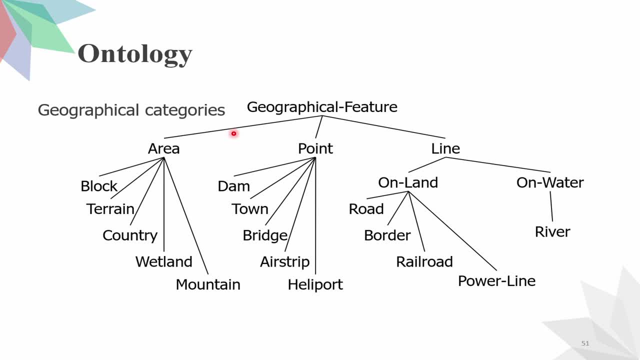 So which represent the detailed knowledge, some detailed knowledge of that particular field. Okay, if I am talking about the particular field, that is computer science of engineering. So there are many courses in computer science of engineering, There are many subjects in computer science of engineering. 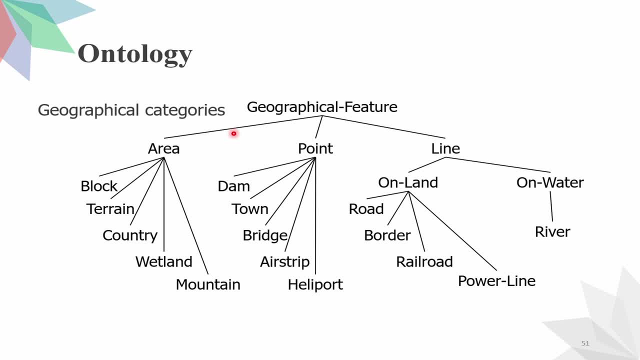 For example, we are learning object-oriented concept, we are learning operating system. we have a database management system. Now, if I will do detailing in database management system, then there are many more concepts in which you have relational database management system. there are normalizations. 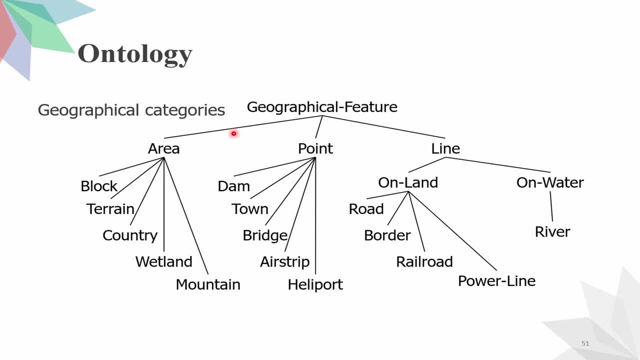 So there are many concepts. So whatever information you have here, the information is divided into three categories: one is top-level, one is general-level and one is domain-specific. That means, if I talk about computer science and information technology, then that is the domain-specific knowledge. 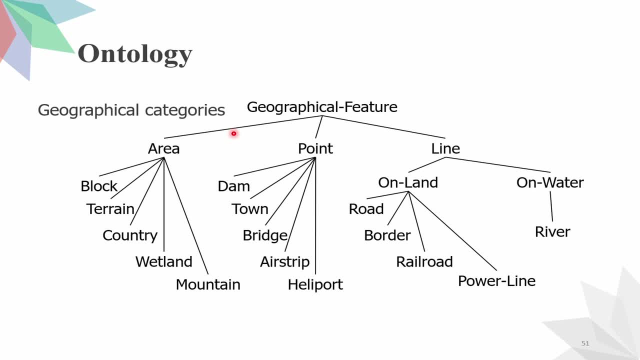 Now, what is its work in knowledge representation? In knowledge representation, similarly, we represent data only or we represent knowledge only. So whatever our knowledge is, we can categorize it in top-level, general-level and domain-specific level. So this information. 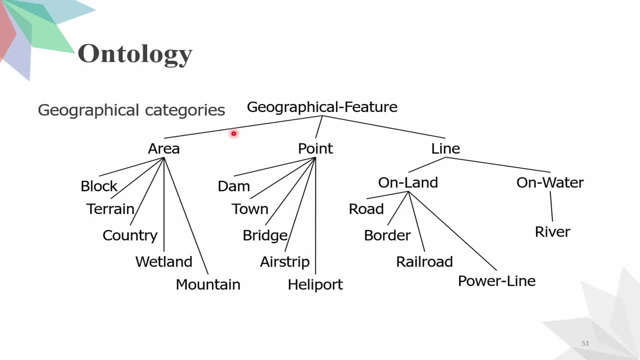 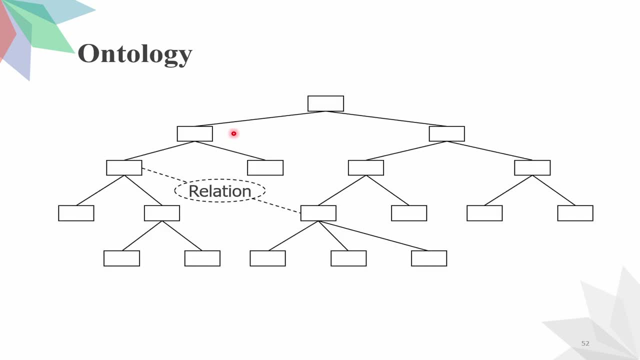 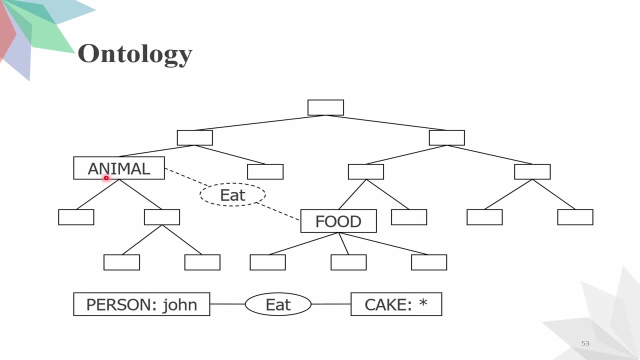 if we want to develop a knowledge base and if we want to represent knowledge in it, then how will we do it? It describes the ontology. So in ontology we also have to represent the relationships between the different objects and entities. Let's suppose we have an animal. 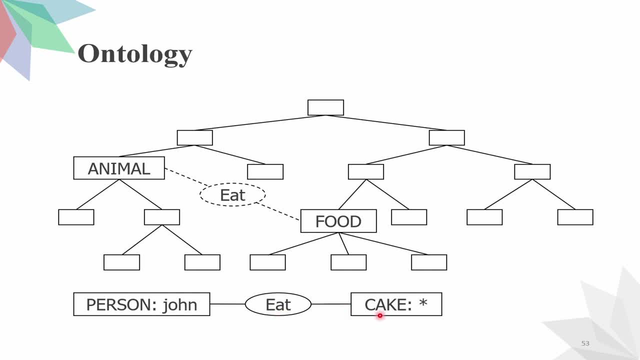 Animal eats food Person John ate cakes. So this is nothing about the relationships of ontology. Ontology is your philosophical concept, in which you detail your abstract information, In which you have representations, naming, conventions, entities, concepts, objects. 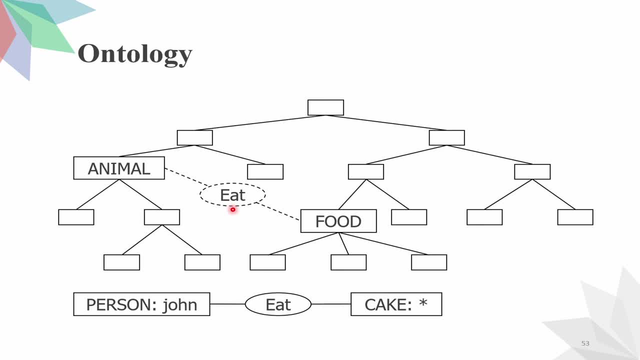 relationships between objects, interrelationships, hierarchy- all these details are there And ontology is a formal definition And if we look at it from a physical point of view, when we represent knowledge, then we need all these things in knowledge representation And knowledge representation. 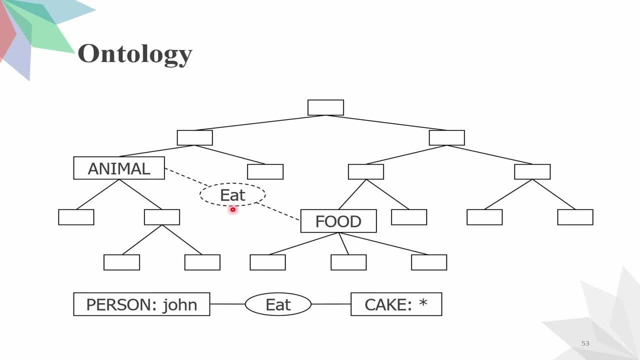 when we represent knowledge, we need to detail: top-level information, middle-level information, domain-specific information. Whenever we represent knowledge, how do we represent the knowledge we have? That type of study is called as ontology. Okay, That's all from today's topic.